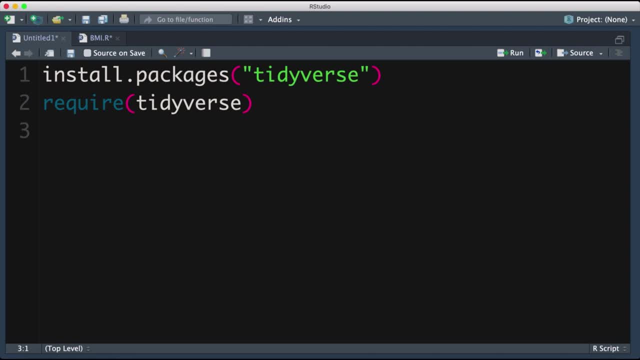 code. So, firstly, if you want to see a list of all the data sets that are existing in R, that are already there for you to use and practice with, just push data, open brackets, close brackets, command enter and there's your list. Now there are some data sets that come with packages, So 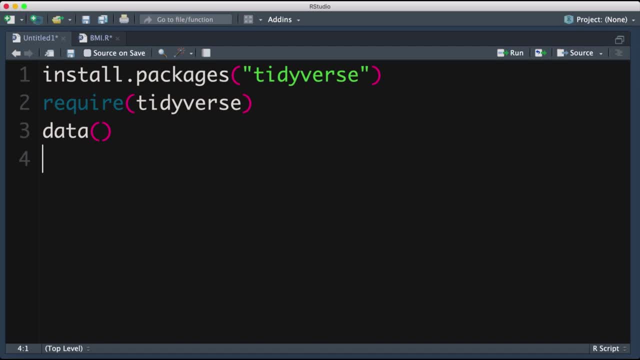 once you've installed the Tidyverse package, you get additional data sets, one of which is the Star Wars data set, And we're going to have a look at that today. So let's have a look at the Star Wars data set. 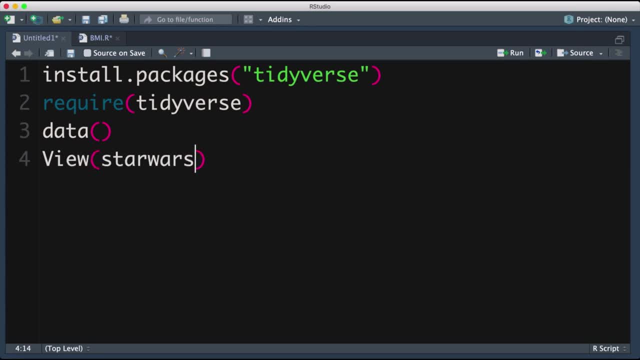 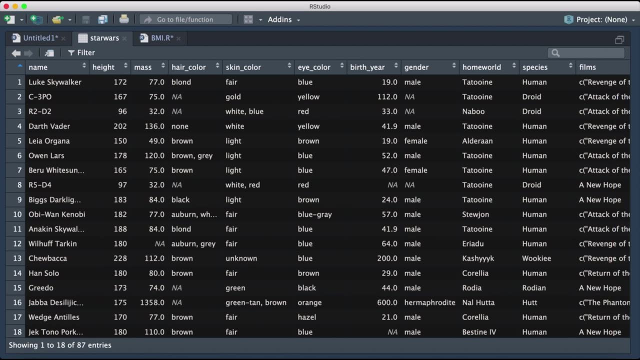 Type in view Star Wars, and there's the Star Wars data set, So we're going to do a simple analysis here. I'm a medical doctor, so I'm interested in how healthy the various characters in the Star Wars movies are. One of the ways, as doctors, we look at health is we look at something? 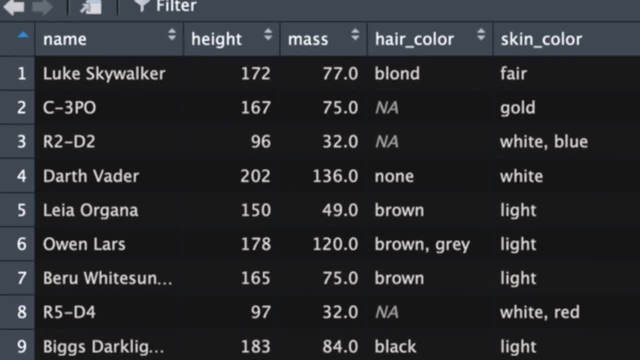 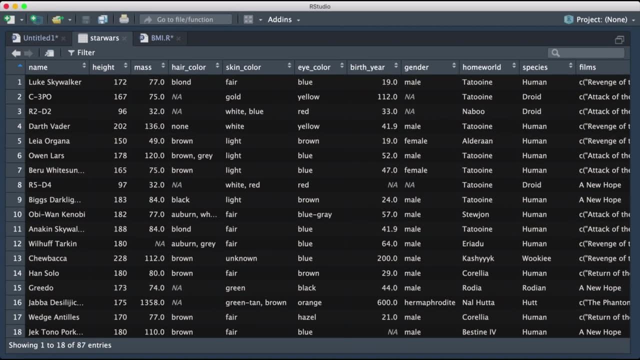 called the body mass index. And to calculate the body mass index we take the mass in kilograms and we divide it by the height in meters squared and we get a body mass index Right. and we could ask the question: is the body mass index different in males or females? 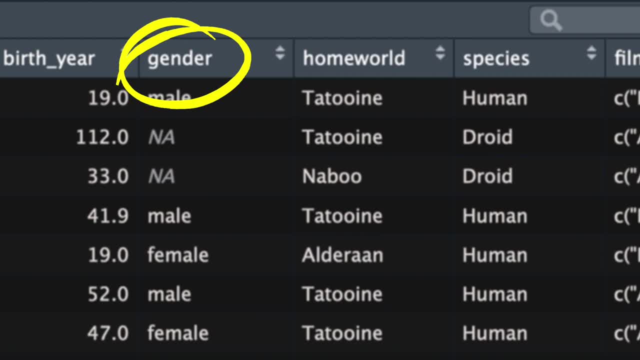 Right. so we've got gender here, so we want to look at height, mass, gender and we might want to say we just want to stick to humans because we don't think droids will have a significant body mass index or anything meaningful there. Okay, so let's have a look at how we would do that. 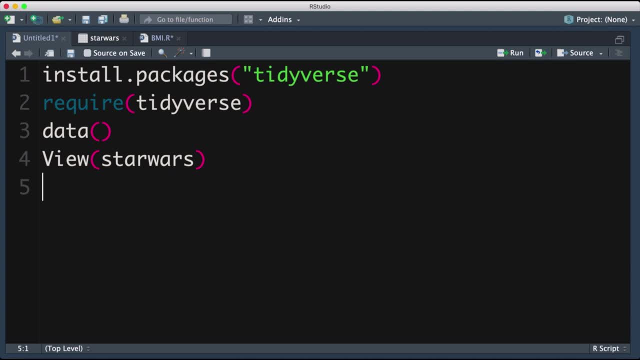 Okay, we're going to tackle this data set the Tidyverse way and we're going to use these things called pipe operators, And I've talked about them in a previous video. but they're very easy to use, It's very intuitive and it allows us to string together the Tidyverse vocabulary. 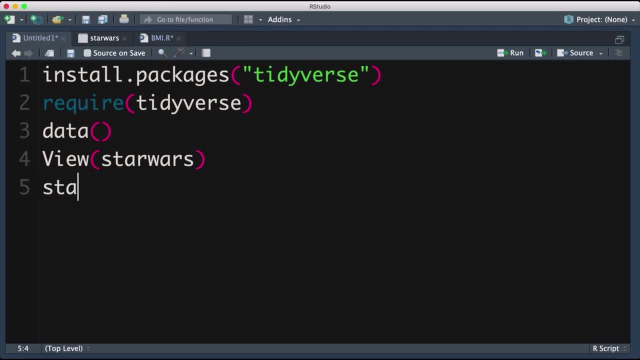 Okay, we start off by saying we're working with the Star Wars data set And then we put in our pipe operator and the pipe operator. if you don't know what it means, think of it like this: It means, and then So we take. 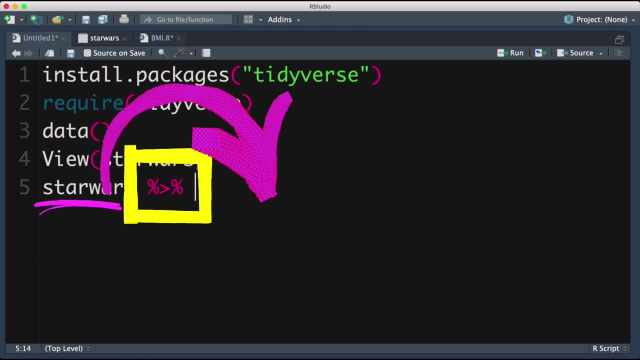 what's on the left-hand side of the pipe and we pipe it into the right-hand side. We're going to do it on separate lines. I'm going to go to a new line after each pipe operator, but Ari's going to think of it as one long, continuous line of code and it's going to run it all together at once. 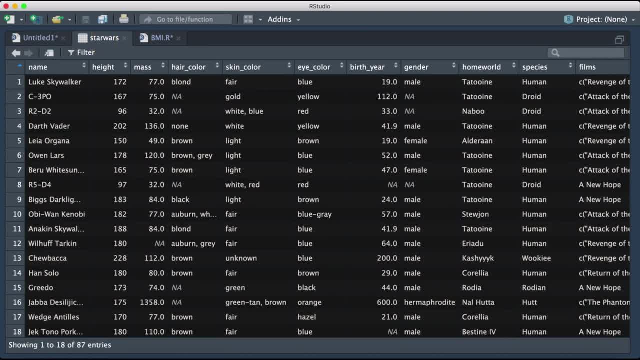 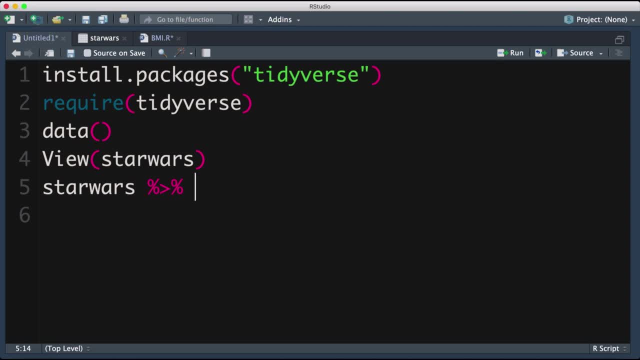 Now the Star Wars data set has got lots and lots of variables. We only want to work with a handful of variables. We want to show you that types of variables can work. So what we're going to do is we're going to simplify our lives and make things a little bit easier by selecting certain 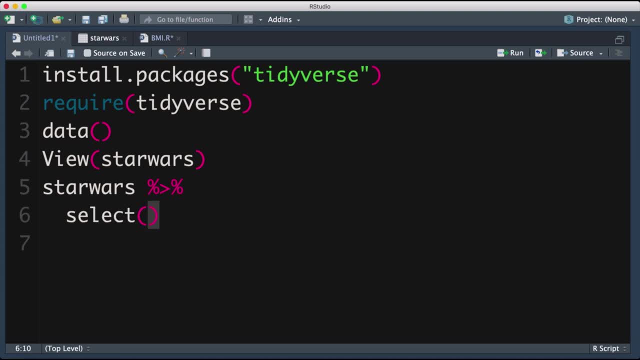 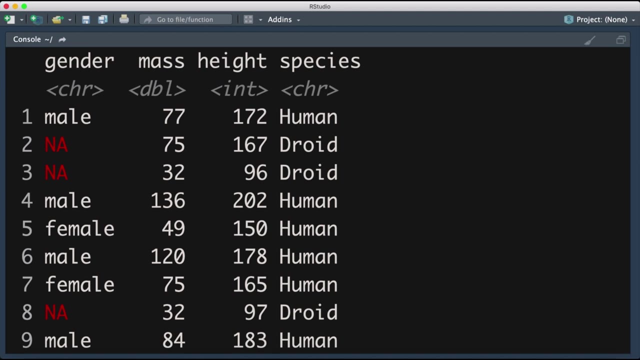 variables, And it is literally that easy. We type in the word select open brackets and we type in the variables that we're interested in: Gender, mass, height, species, push Command, Enter. Okay, so we can see R has produced now a much smaller and more manageable data frame. It's only got the four. 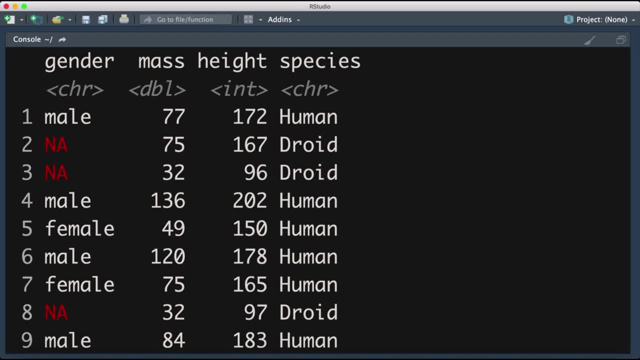 variables that we're interested in filter out anything that's not a human right. So droids aren't of interest in this particular analysis. So let's do that right. We're back at our source. Again, we put in our pipe. operator. 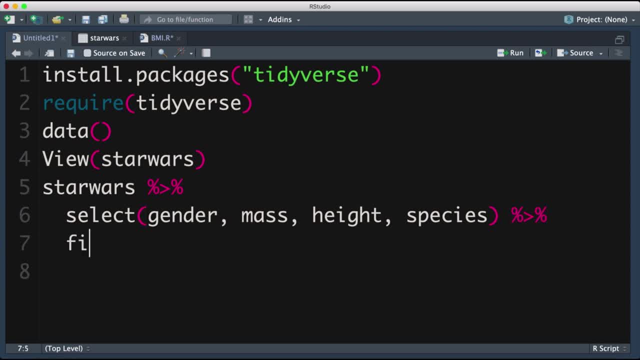 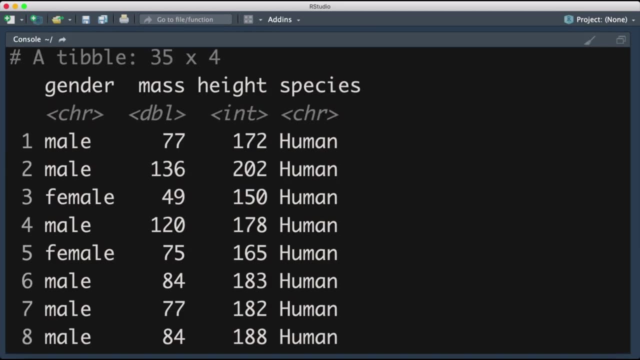 which is shift. command M. go to the next line and let's type in filter. We want our species to equal to, equal to and human, And we use the double equal to's because we're asking a question. Command enter And we've got gender, mass, height. 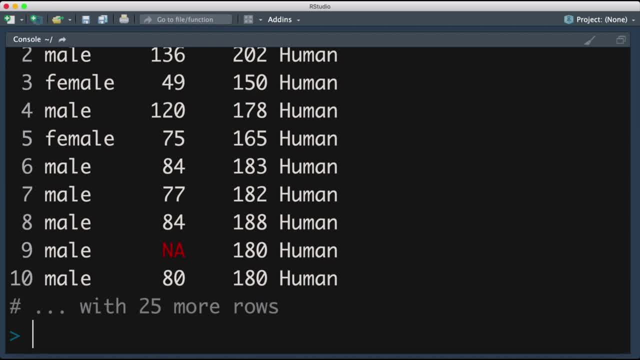 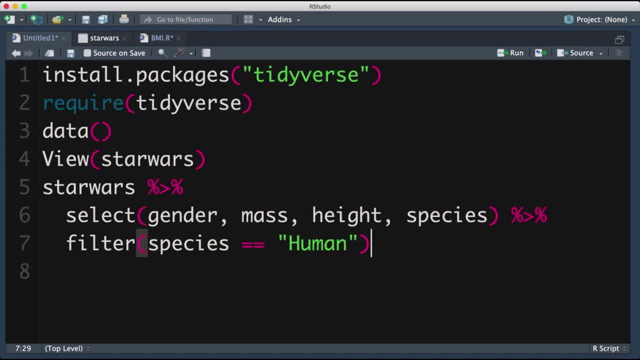 We still have an NA here and I'm not sure why that's there, but we don't want it. So we're gonna say NA omit and get rid of it Now in this video- I'm not gonna get into the science behind when you do and don't use NA omit. 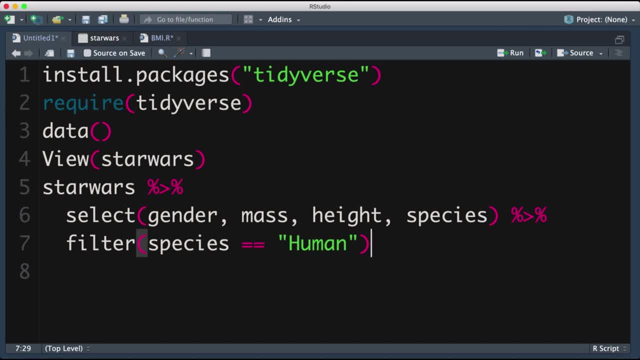 when you do and don't remove rows that have missing values. I'm really just trying to teach you how to use these pipe operators and how to use these functions, So let's not worry about that too much. Let's stick in a pipe operator for argument's sake. 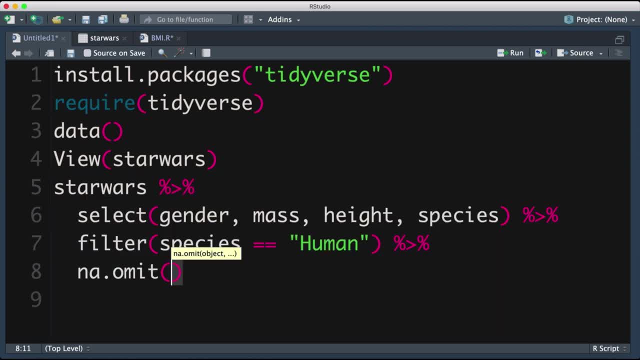 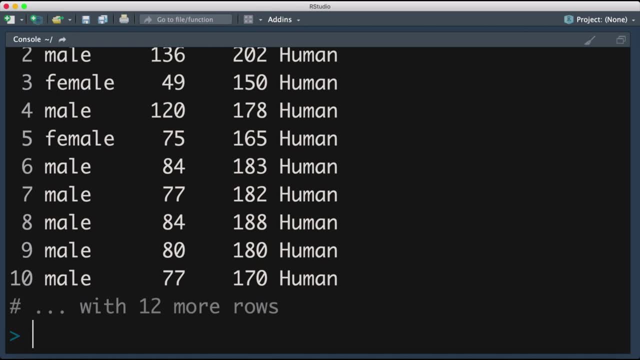 and say NA omit, and just open brackets, close brackets, push enter, control enter and you'll see that that missing value row is gone completely. There you go. gone. Shift control one. to go back to the source. Now we wanna create a body mass index. 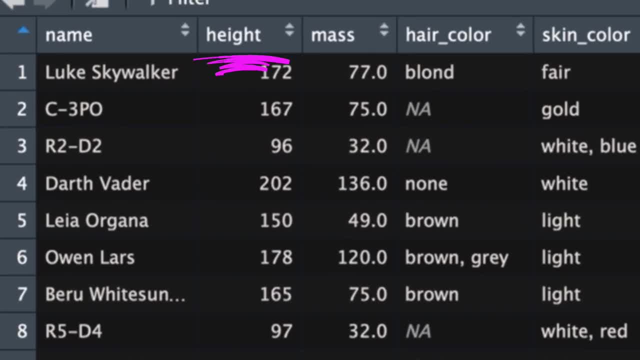 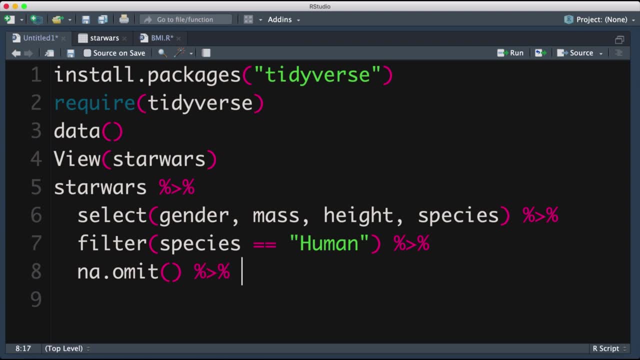 but you'll notice, if we look at the data, that our height is in centimeters and we need that to be in meters. So we wanna change that variable a little bit. Let's do that. We're pushing a pipe operator and now we use something called mutate. 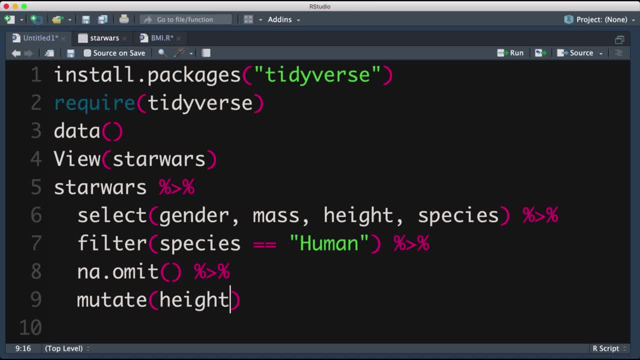 Okay, open brackets. We type in height, right, We create. we could be creating a new variable now, but what we're gonna do is we're just gonna basically tell it to change height. So we say: height is equal to height divided by 100. 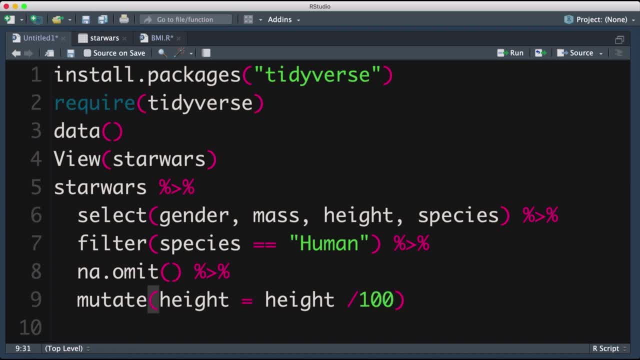 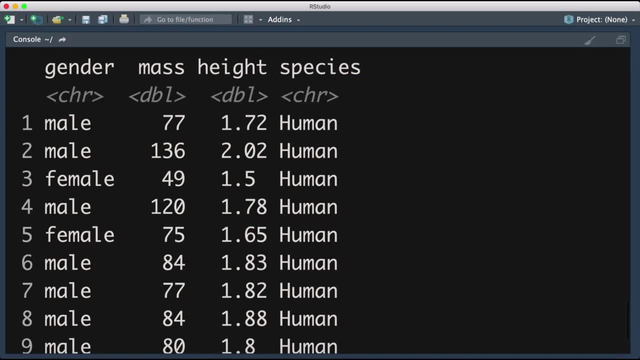 Now you'll notice I didn't use the double equal to's. We're not asking a question, but we're telling R to change height and make it equal to what height was, but divided by 100. And we can see that the height is now no longer.